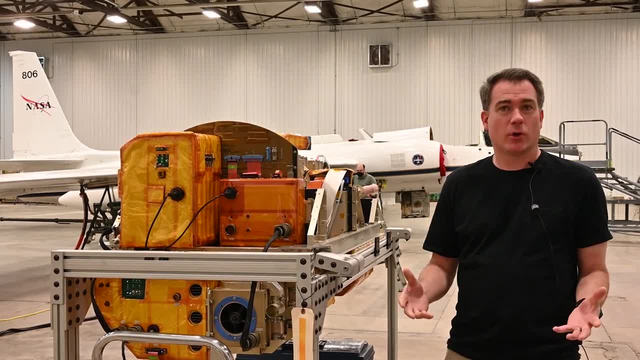 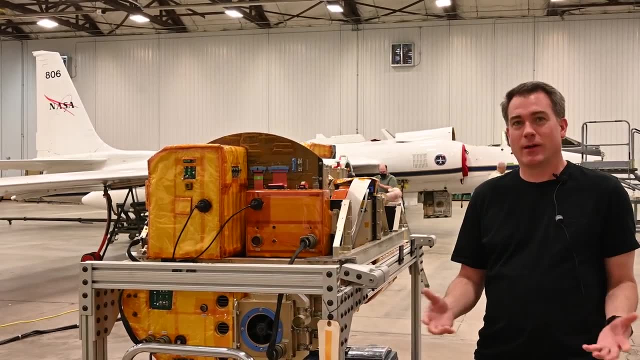 bromine are well known to destroy ozone. So one of the reasons we're interested in measuring chlorine and bromine is we want to make sure that we understand the chemistry so that we understand ozone. And so every year there's these seasonal ozone holes at the poles and 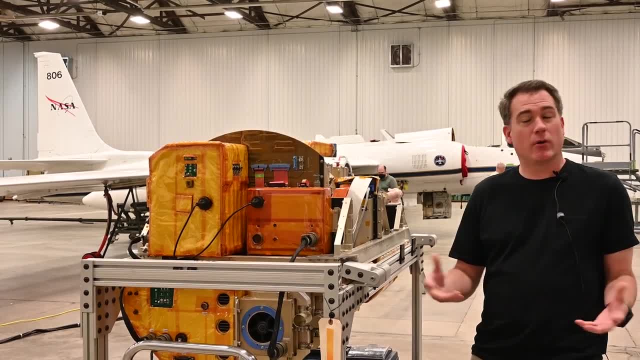 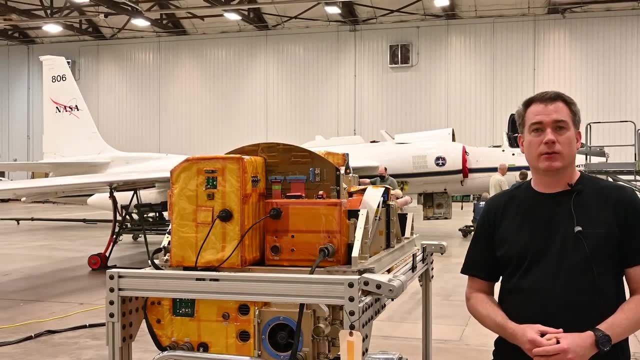 the holes which I think everyone is familiar with, But chlorine and bromine are everywhere in the stratosphere, And so we're measuring it over the mid-latitudes this summer as part of the DCOTS campaign, And one of the things we're interested in is this process of convection. 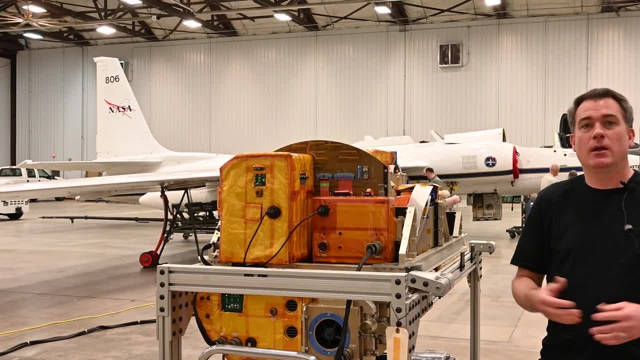 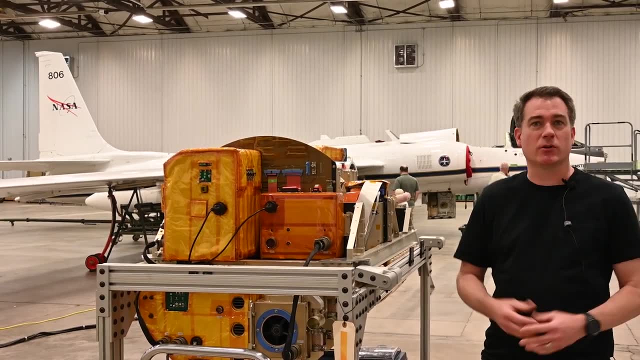 that brings air up from the troposphere into the stratosphere, It bypasses the sort of normal way the atmospheric circulation works, And so if we're bringing tropospheric gases into the stratosphere, does that potentially have an impact on the halogen chemistry And 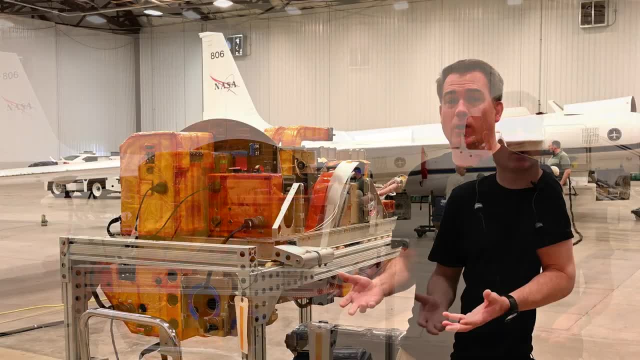 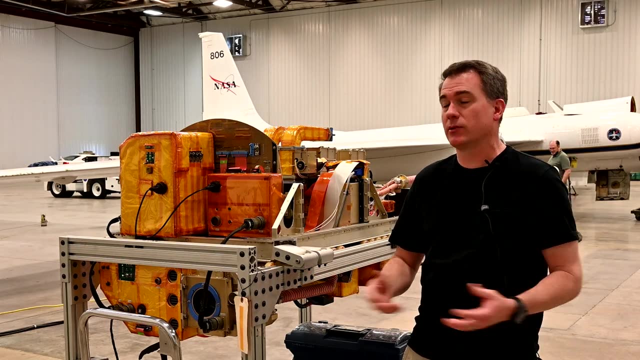 also with the water vapor that we know for sure comes up with these convective processes. is it possible that the chemistry of the stratosphere is impacted that way as well, through heterogeneous reactions? And so that, in a nutshell, is the reason why we're interested in halogens. So, specifically, most of the halogens that make it to the stratosphere come up in the organic form, which means they have carbon in them, But then it's converted into inorganic chlorine once it's in the stratosphere. Inorganic chlorine in the stratosphere are HCl, hydrochloric acid, chlorine nitrate. 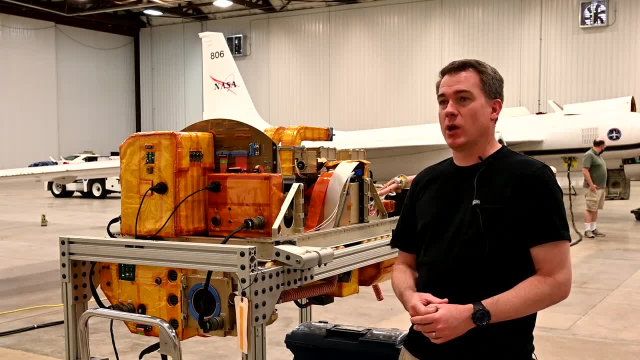 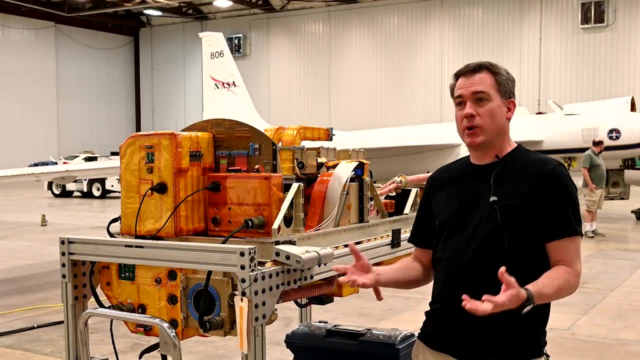 and ClO. So we're measuring two of those three And we also have a way to figure out the total amount of inorganic chlorine, so we can actually calculate the HCl, the one we're not measuring. So we do have a pretty complete picture of what's happening with the chlorine chemistry. 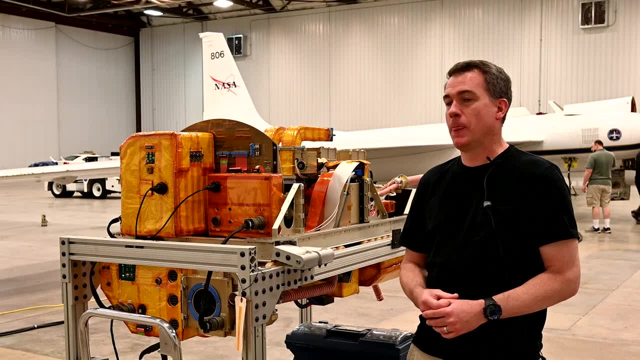 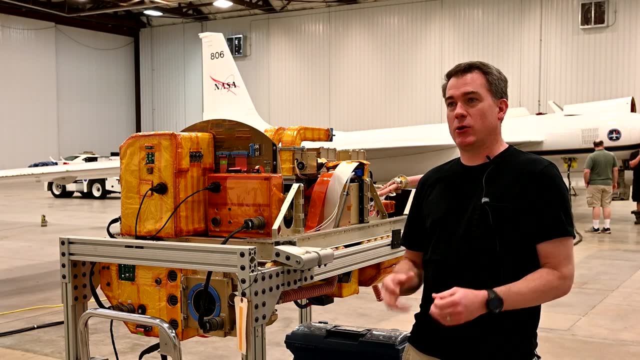 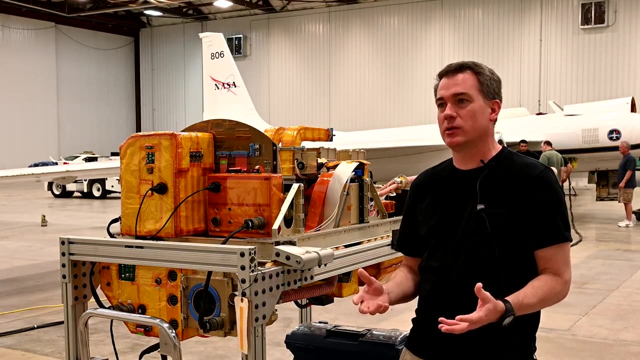 over the US in the summer as part of this mission. That's one of the goals- And also for bromine chemistry, BRO, the molecule that we measure is the most significant inorganic bromine molecules. So, again, these compounds that we're measuring are present at very small concentrations. 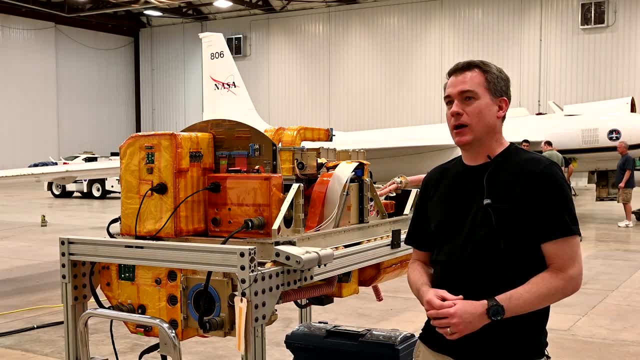 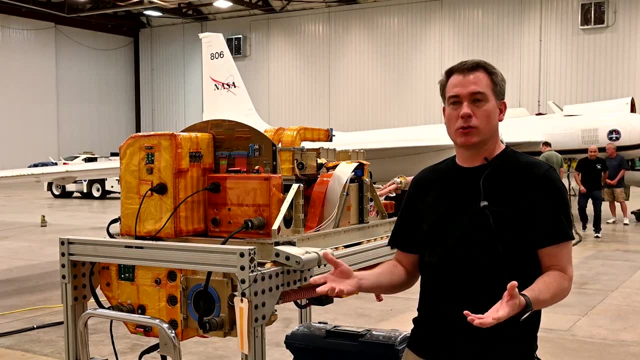 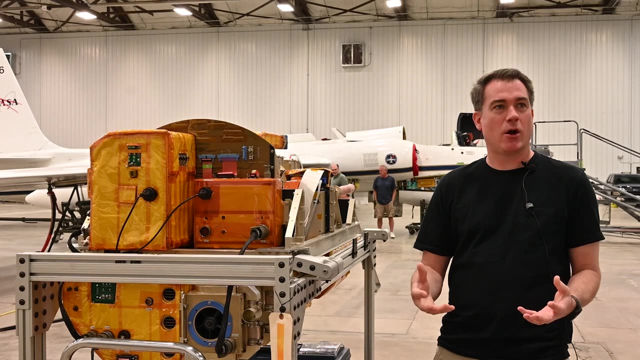 so parts per trillion units, which is very, very small. But because of the way the catalytic reactions work, a single chlorine or bromine could destroy many, many thousands of zones. So that's the reason why we care, even though they're present in very small concentrations. 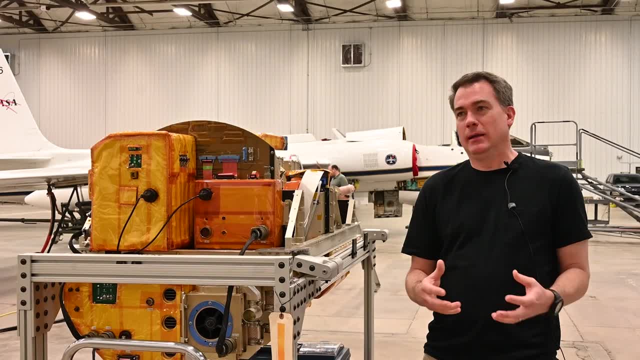 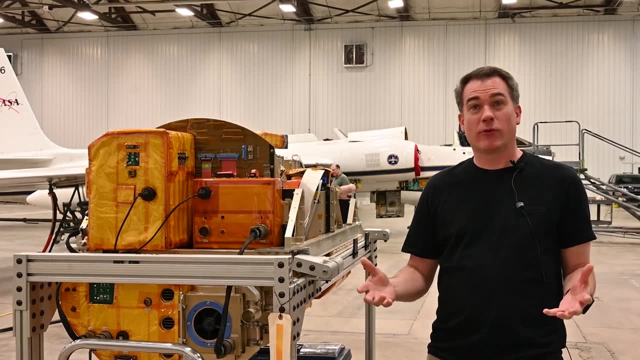 So if we go back in time to think about what things were like in the mid-19th century, we know that in the mid-1980s everyone was using CFCs, chlorofluorocarbons and all sorts. 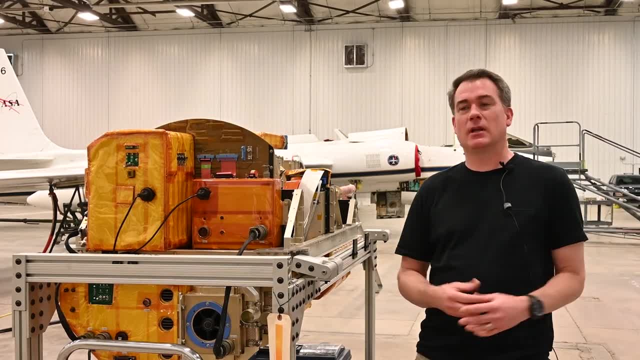 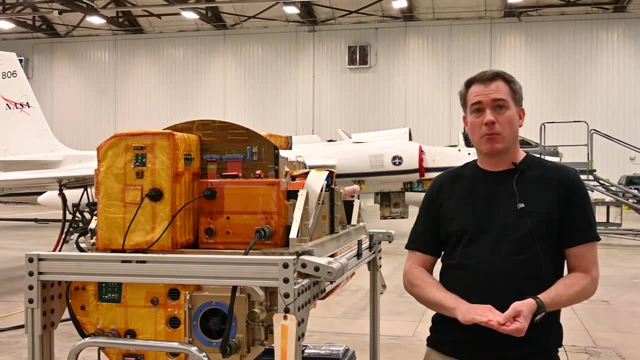 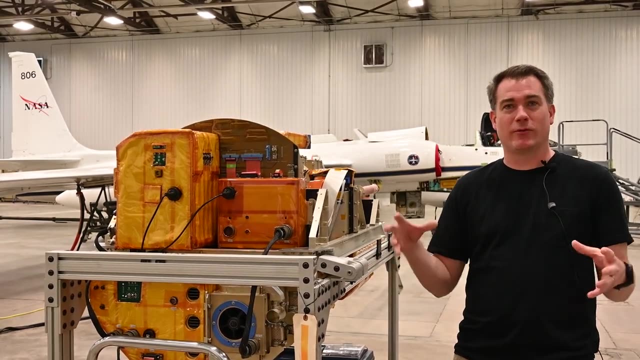 of deodorants and sprays and refrigerants And people realized that that was actually leading to ozone destruction. So those things began to be phased out as part of the Montreal Protocol, which was this international agreement, the most successful international agreement in history. All nations on Earth have now agreed to limit their use of chlorofluorocarbons. 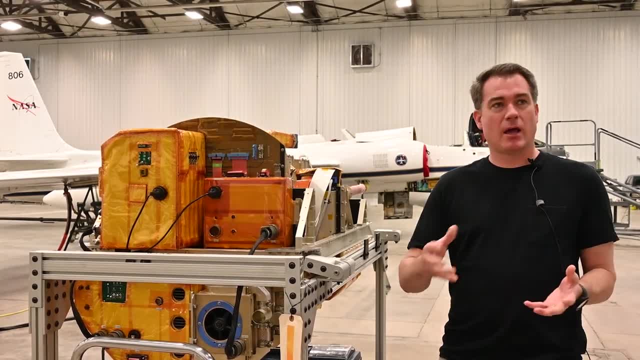 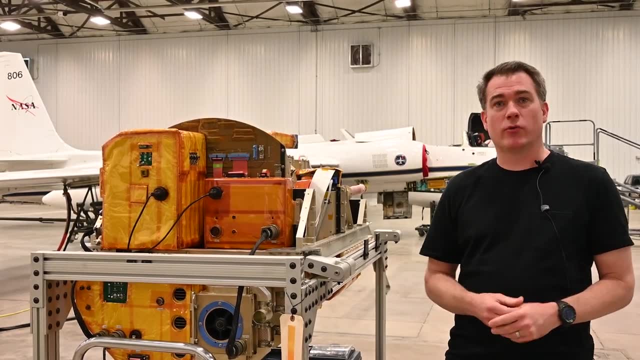 And also halons which contain bromine, And so as part of that, slowly over time, we are seeing the amount of chlorine in the stratosphere go down, And we'll continue to see that over time. But one of the other things we're able to do in this mission is to actually take. 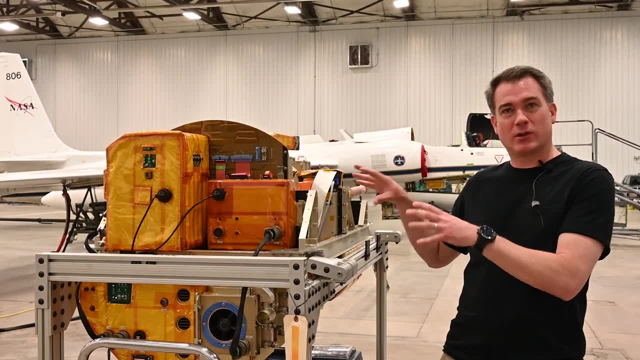 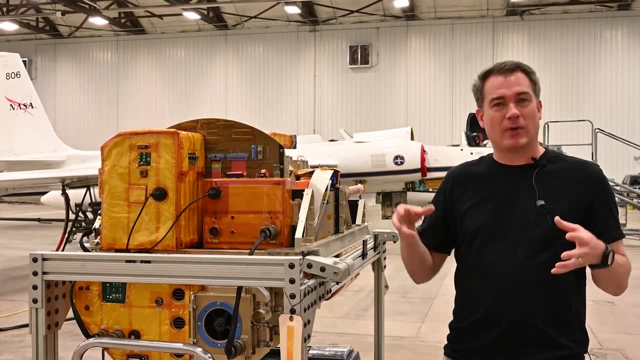 a look with this in situ payload. So in situ means we're actually measuring right in place as we're flying through. So we have satellite measurements of these. but satellites are limited in terms of how detailed and specific they can actually determine the concentration. 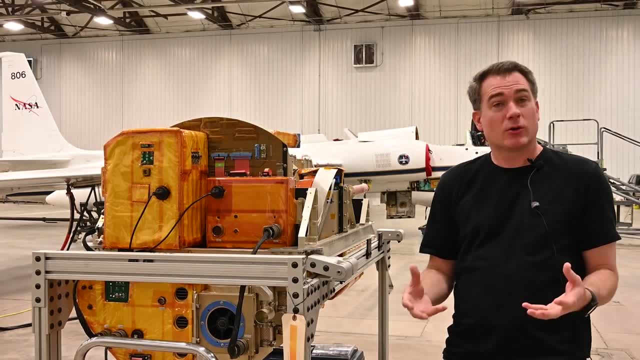 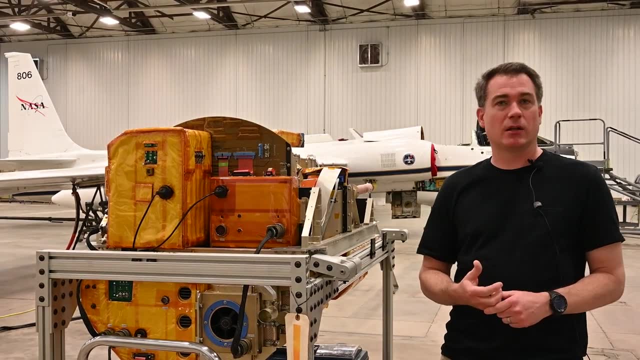 But to look very carefully at what the inorganic chlorine concentrations are in the stratosphere right now with a precision that's not possible from a satellite instrument, And this is the first time this has been done in quite some time, So it's very helpful to do that. 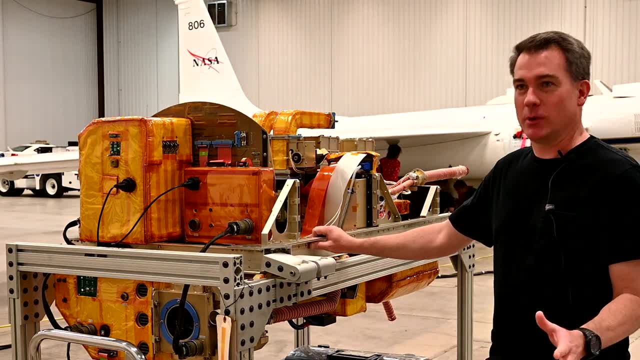 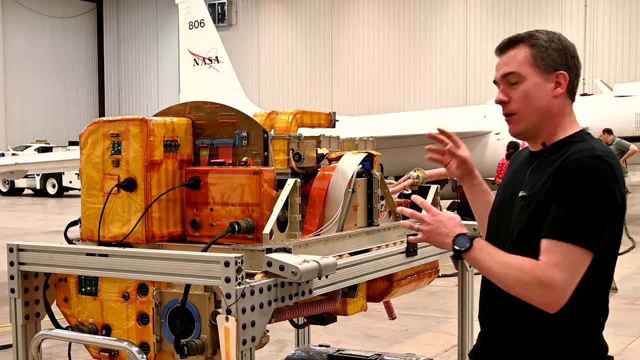 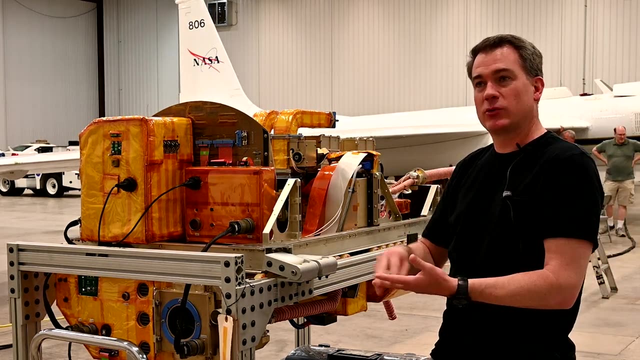 Okay, so this instrument is called the Harvard Halogen Flight Instrument. The way we detect CLO- I'll just use that as an example first of all- is we add NO, which is nitric oxide, where, as it's going through the instrument, So the nitric oxide reacts with CLO and very 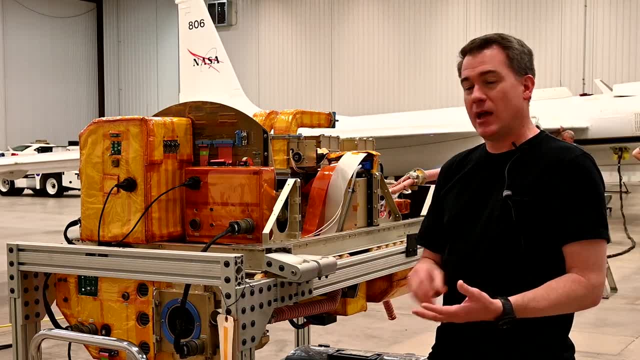 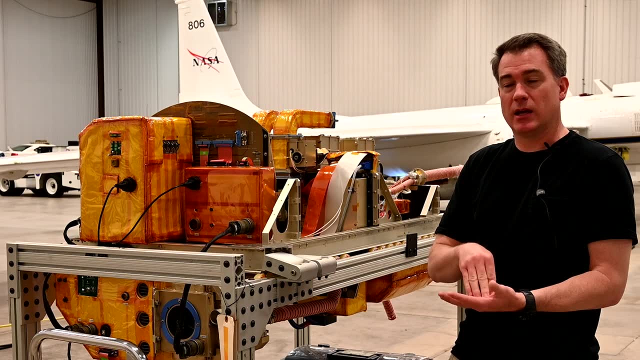 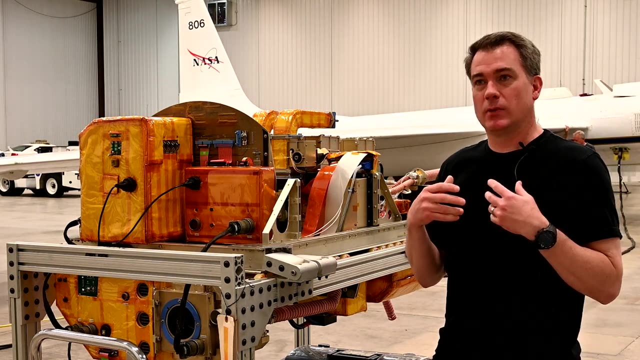 rapidly converts it into chlorine atoms, And so we actually detect those chlorine atoms by a process called atomic resonance fluorescence. So there's a vacuum ultraviolet light source that we actually make ourselves that excites the chlorine atoms in our flow ducts and then those fluoresce So they emit light as the excited chlorine atom relaxes back to the 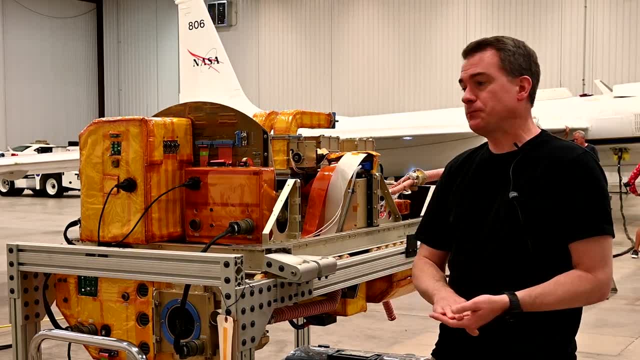 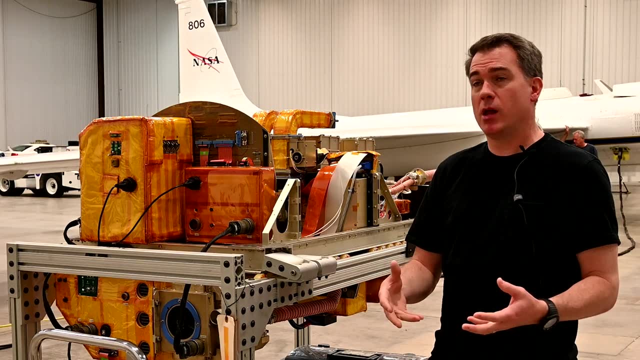 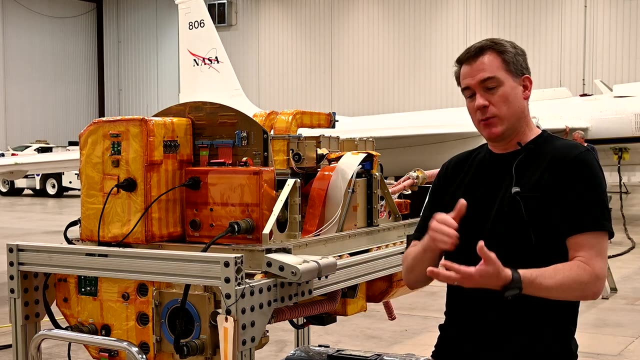 ground state And we detect that light with a PMT And so by titrating with NO we can determine how much CLO is there. For chlorine nitrate, which is a larger molecule, we heat it up very hot: 220, 230 degrees Celsius. We break. 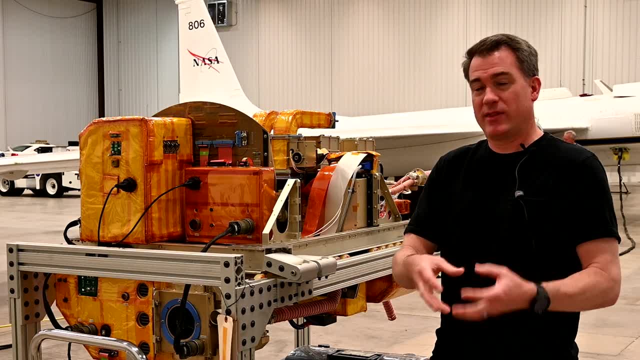 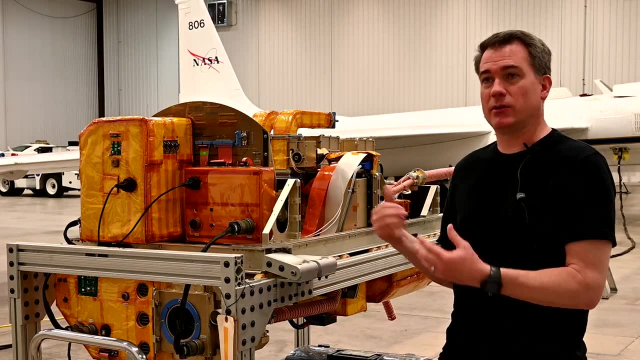 the CLO-NO2 bond. And so with that CLO fragment of the chlorine nitrate we titrate that with NO And by the same process as the ambient CLO we convert that to chlorine atoms and we detect those chlorine atoms. 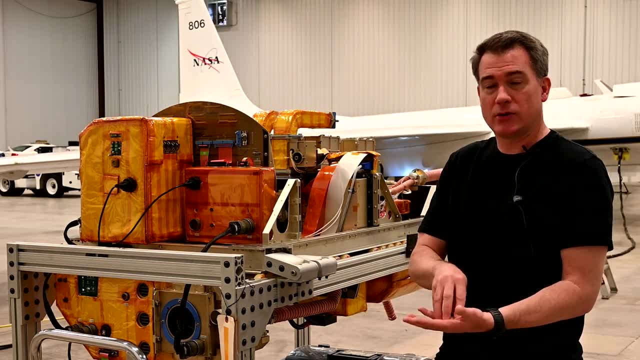 So basically, by modulating that with NO, we can determine how much chlorine nitrate is there. By modulating temperature and the amount of nitric oxide we're adding and detecting chlorine atoms. we can determine the amount of CLO and chlorine nitrate in the stratosphere. 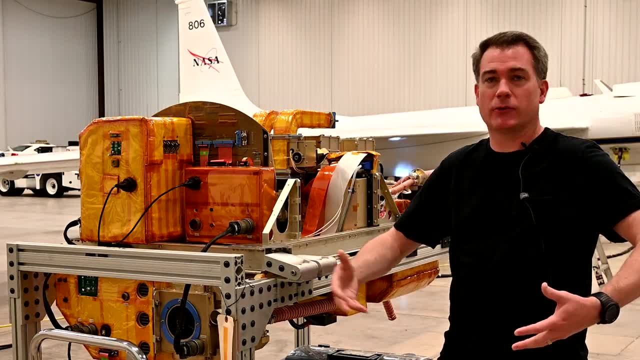 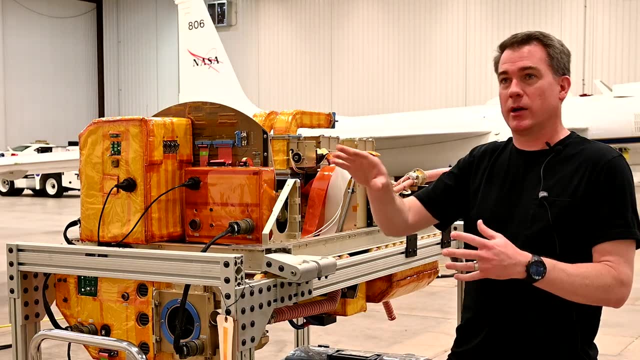 So this instrument flies in a very large- it's called a super pod. It's a big cylinder that sits underneath the left wing of the plane. The air. so the plane flies along and the air as the plane's flying along goes right through our instrument up and out, And we 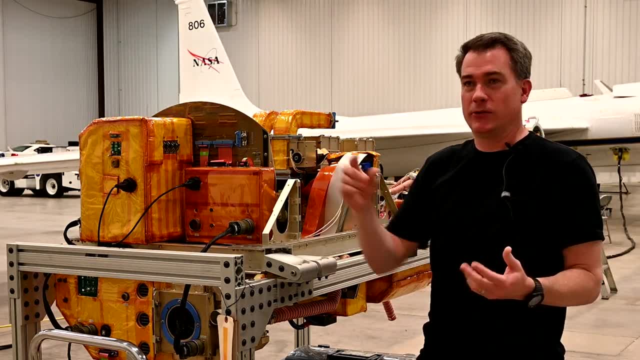 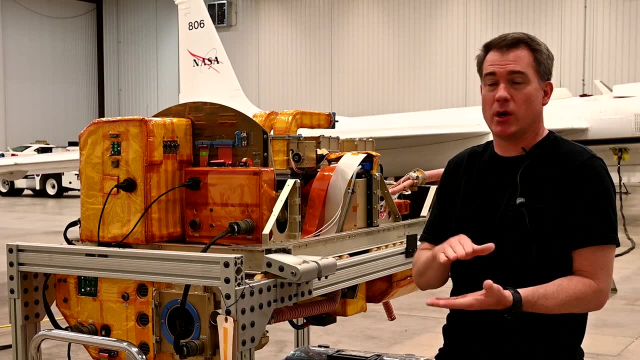 have about 10 milliseconds to make this detection, as the instrument's going along, And so that's how we do it. And so for bromine, similar process For BRO. we also titrate with nitric oxide and detect the bromine atoms. It's a similar atomic resonance, fluorescence. 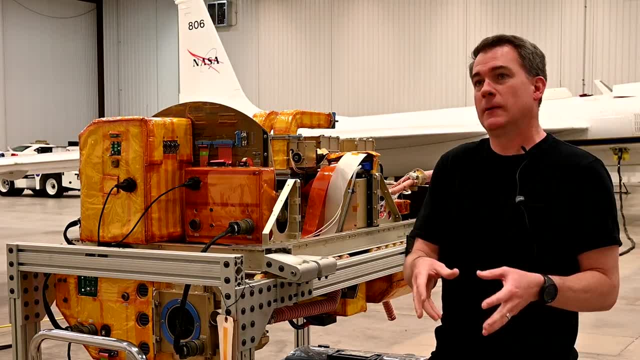 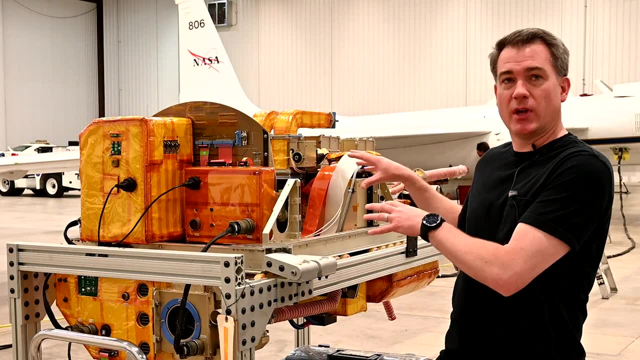 technique. The difference is we have a different light source that's tailored for bromine And we change some purge lines, But other than that it's a very similar detection technique. So this instrument has four different detectors And, depending on how we set it up with our 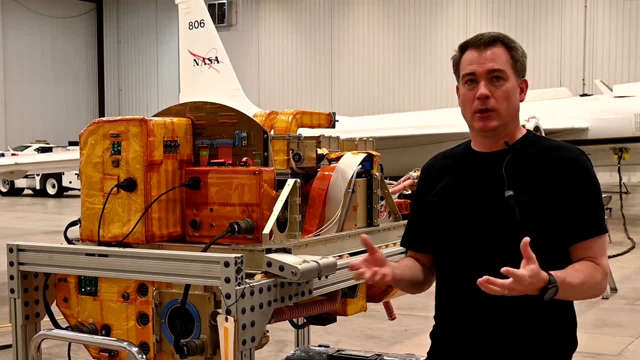 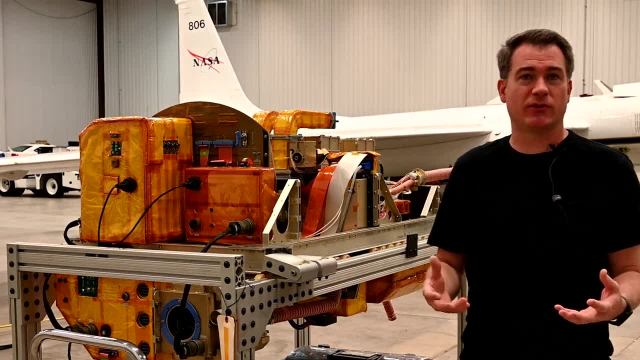 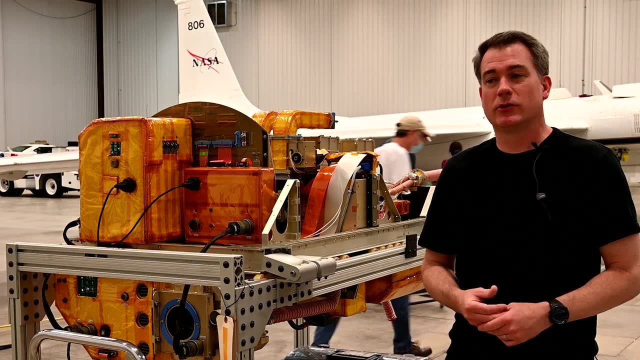 this instrument over the polar vortices. there's another molecule called CLO dimer or chlorine peroxide, that's present in very high concentrations. It's unique to the poles, So we only measure it there because it's only present in them when it's very cold and very dark. But this 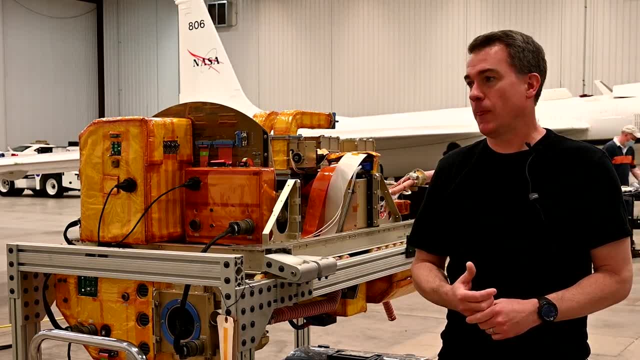 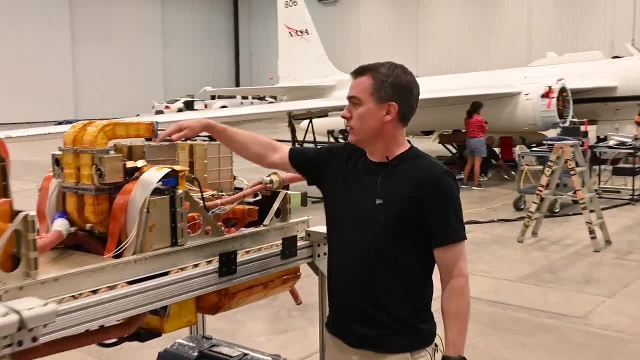 instrument can also measure that as well, And so that's essentially how we do it. It's very simple. So, if you want to catch it in the shot, these are the four different detectors. There's a custom vacuum ultraviolet light source inside of each of these housings, along with quite 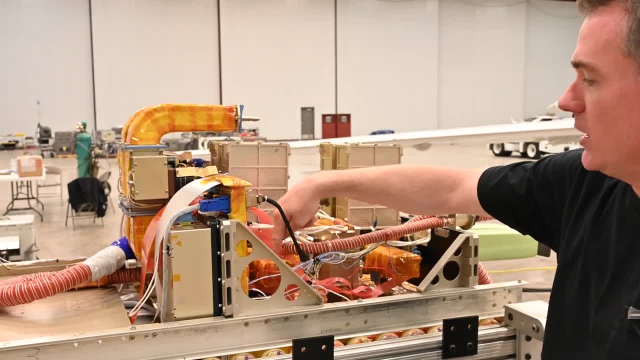 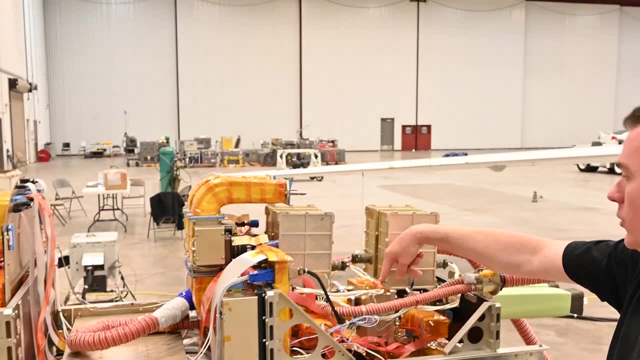 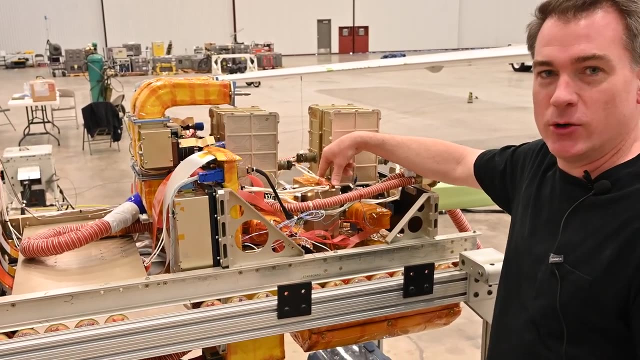 a bit of custom electronics. The detectors are here at a right angle. These are called PMT's photo multiplier tubes. That's what actually does the detection. This here is the dissociation heater. This is a custom part that one might think that having a heater 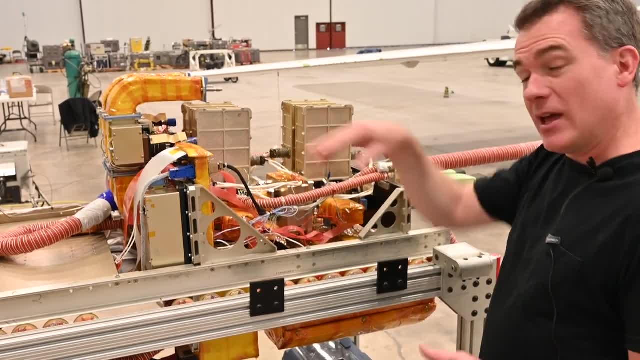 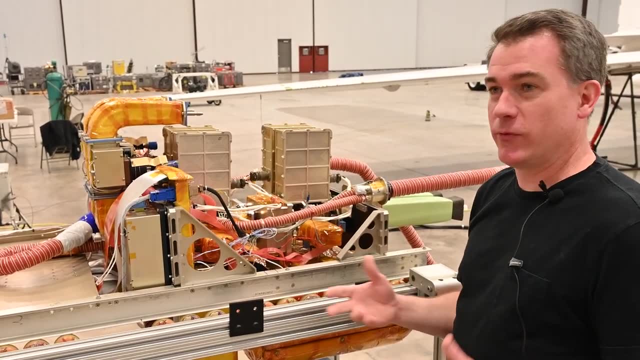 that could heat to 220 degrees Celsius isn't that difficult, and it's actually not to heat it. the challenge is making a heater that's inert, because if you have any sort of metal surface or anything that you might normally think of with a heater, it's 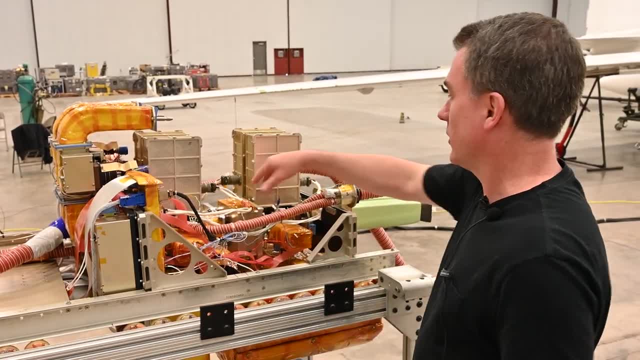 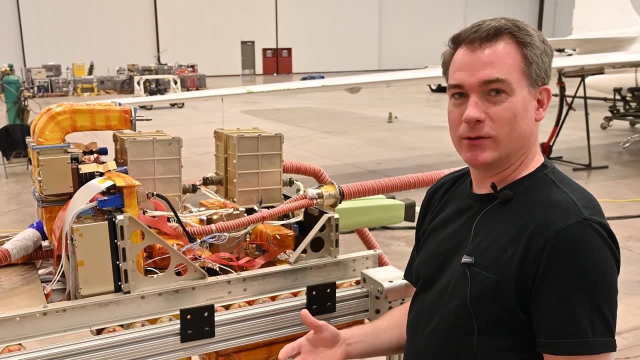 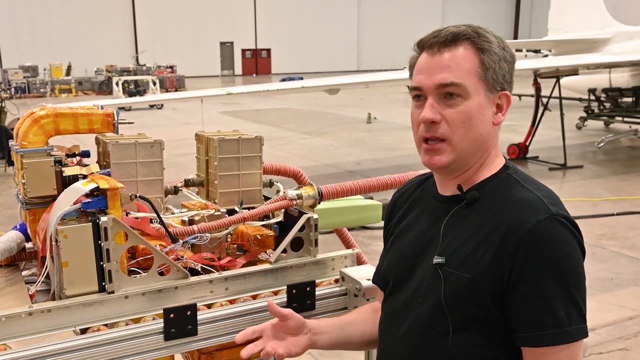 going to destroy the chlorine atoms and impact the measurement, so this is a custom design. you can't see the inside. there's a grid of 28 strips of silicon wafers that we're using to resistively heat up and because silicon is inert to chlorine, and what we've plated the ends of the heater with. 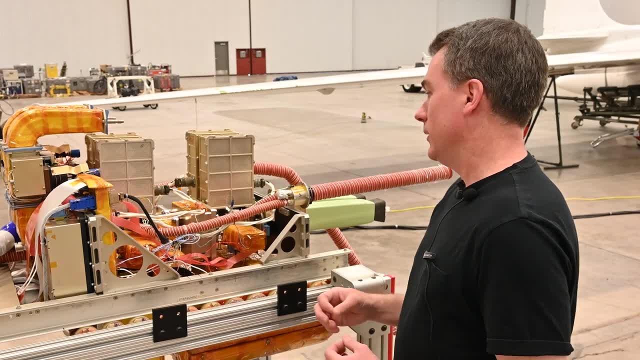 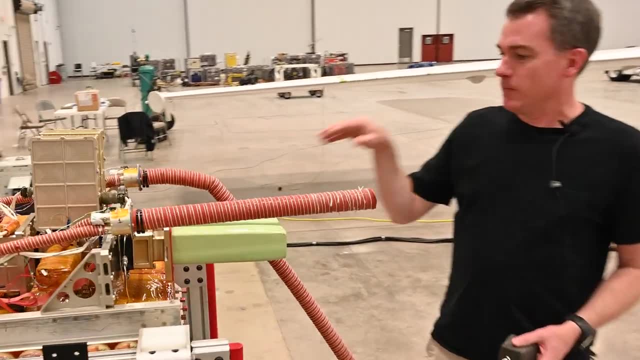 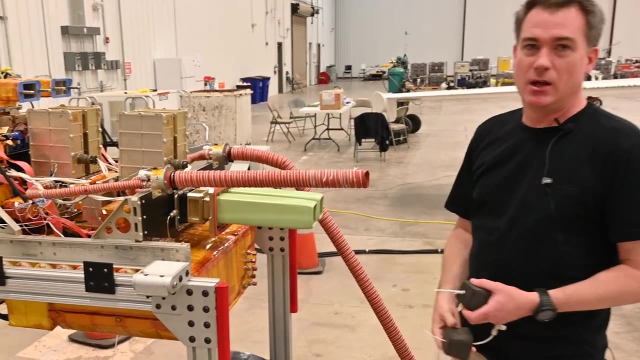 titanium, nickel and gold, they get the electrical connectivity and it works quite well. and these are the inlets in the front. so it's a. it's a double ducted system, so the air is going through and measuring simultaneously in each of the two ducts and again with the four detection axes. we 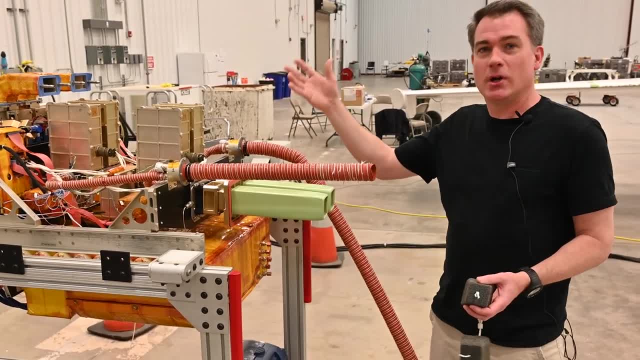 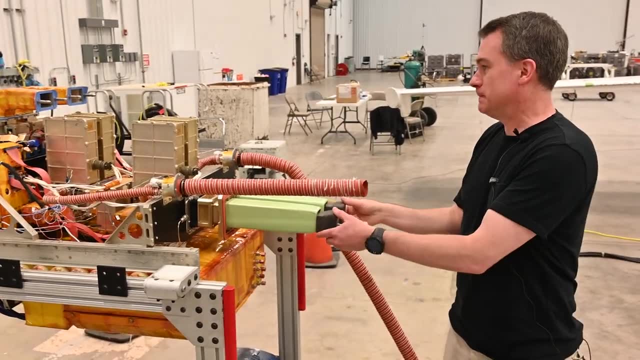 have a lot of flexibility in terms of whether we could measure CO low in four places if we chose to, or we can mix it up depending on the heater and in which lamps we put in. sometimes people will see the instrument, their first reaction as well. what's, what's all this? 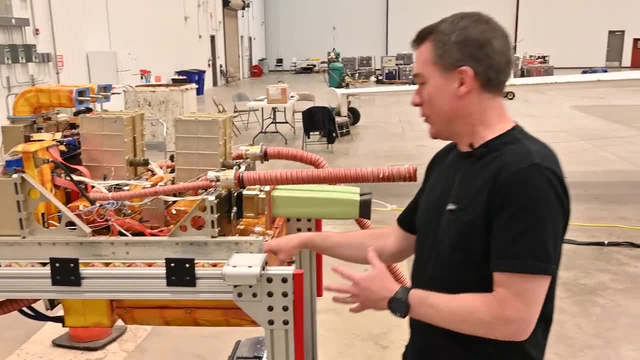 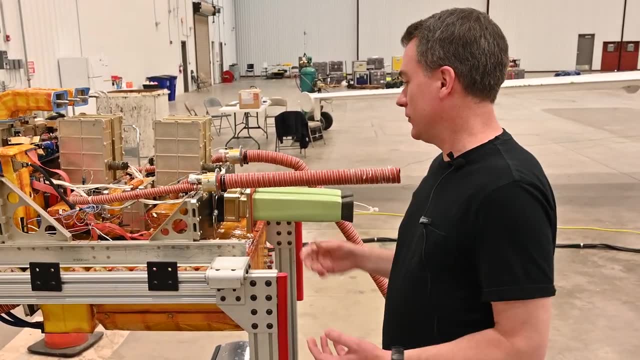 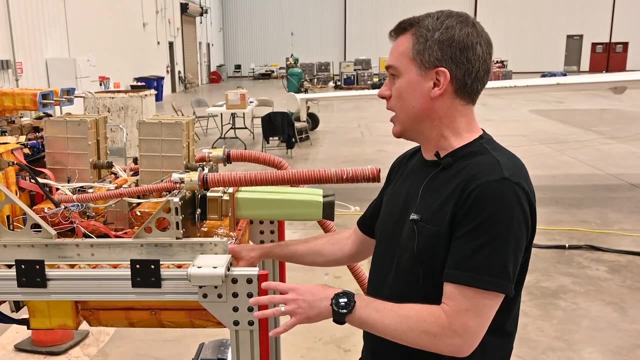 yellow stuff. okay, that's Kapton tape. so the underneath this tape is insulation. it's called Nomex insulation. it's actually primarily used in fire suits, but it's it's very good for flight use. it provides some thermal insulation in the and so the Kapton tape's just a protective barrier over. 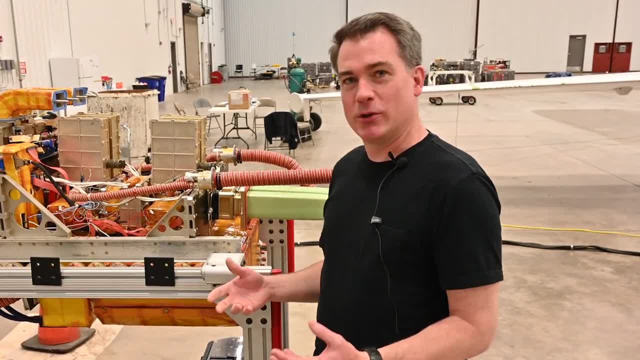 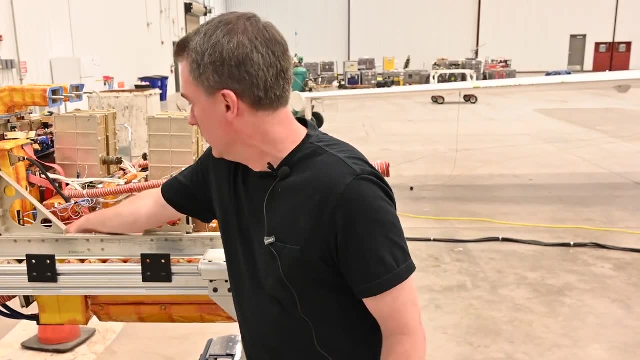 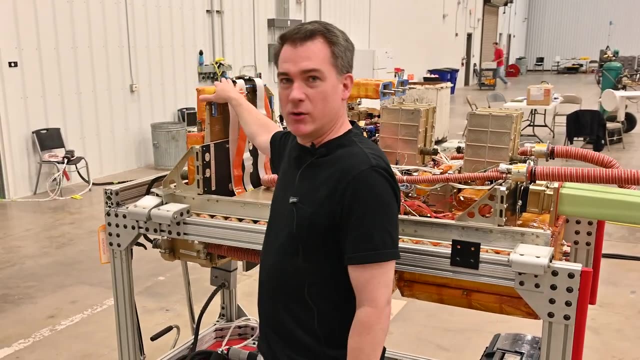 top of that, most of the real intricacy of the instrument you can't see just by looking at the outside. there's quite a bit of custom electronics inside the gas deck and this heater control box and the different housings in the back is a data system that we built that can process all the data in real time. we're actually 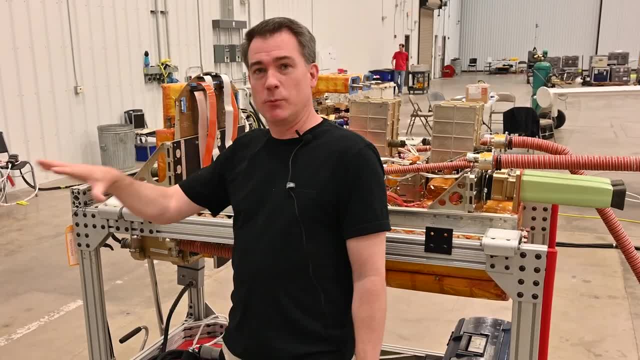 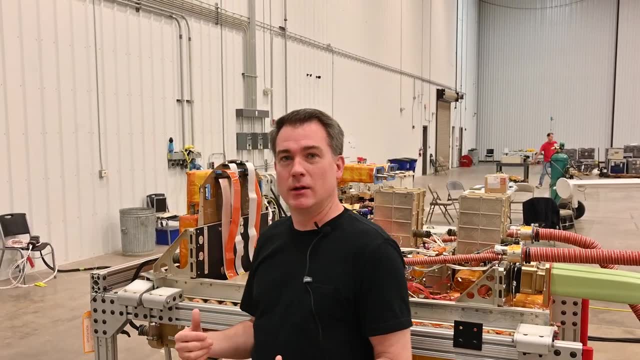 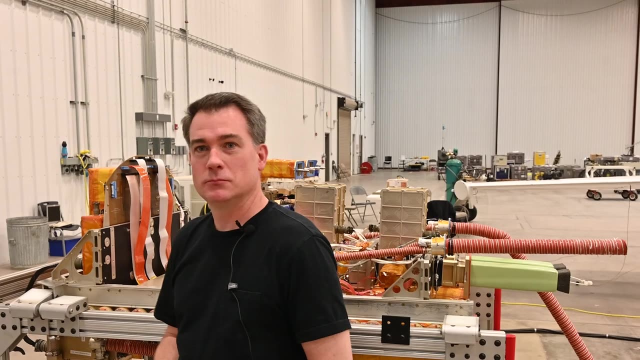 able to send the data down from the plane in real time, so, as the plane's flying along, we get an updated measurement as it, so we don't have to wait for the plane to land to find out how much CLO or chlorine nitrate or BRO we're actually measuring now with with people using less and less, or if